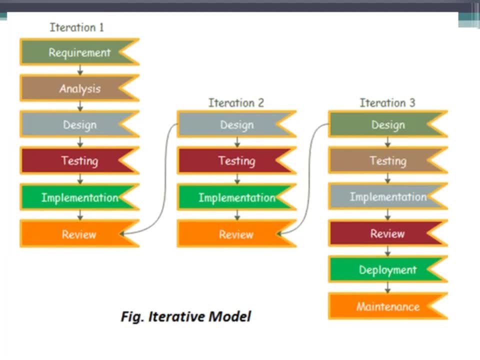 version of the software is created with a new iteration. So basically what we will do: We will start working with some requirements. On the basis of those requirements, we will follow some phases And at the end, we will have a software. We will review this software for its perfection. 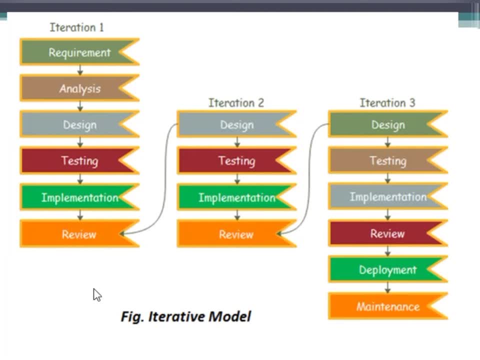 If it is perfect, then this is the final product. If it is not perfect, if there is a need for changes or new requirements have come to us, then what we do is we continue this project in the second iteration and accept the changes in it, incorporate new changes, and then we 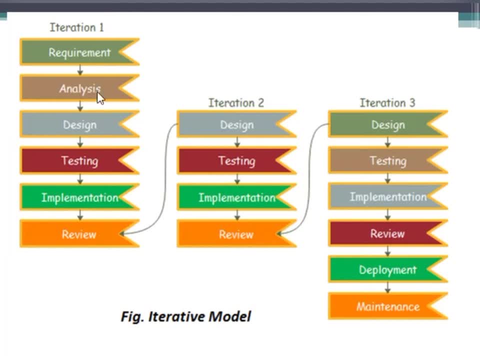 get a new output. So after iteration 1, we will be having the first version of the software. In this first version we will make changes in iteration 2. And after that, when we get the software, that will be the second version of the software. Similarly, all the iterations that will follow. 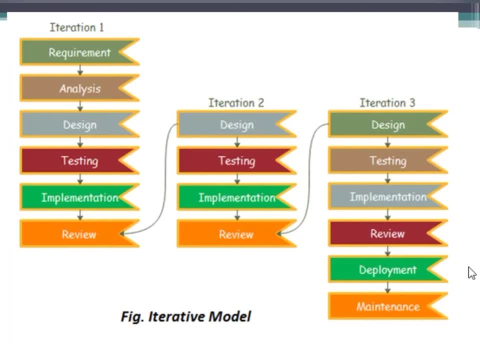 at the end of the last iteration we will be having our final software, which will be the perfect software according to the user requirement. So these are the iterations to make our product, our project, refined. The iterative model allows the accessing of earlier phases in which the variations were. 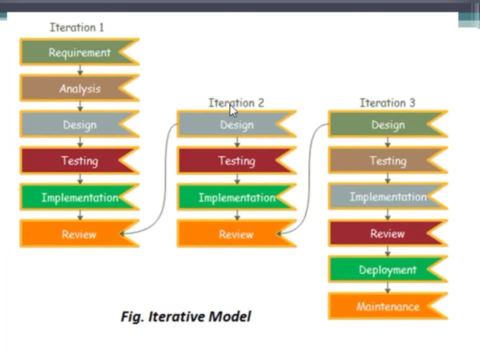 made. If we are talking about iteration 2, then from where will our input be accepted? From iteration 1.. If we are talking about iteration 3, then it will accept the input from iteration 2, and so on. Right, The final output of the product renewed at the end of. 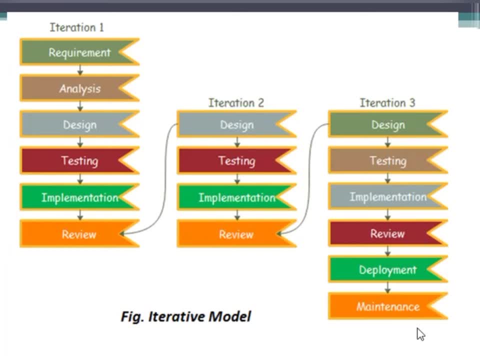 the SDLC. How will we finally judge our product? The final output of the product renewed at the end of the SDLC. How will we finally judge our product? The final output of the product renewed at the end of the SDLC. This also appears to be the final output of the project. 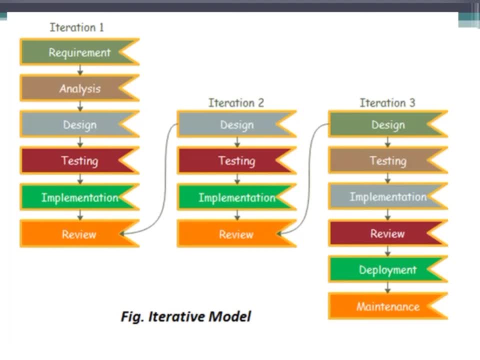 renewed at the beginning of the project. Okay, What are the phases of iterative model? We have similar phases in the waterfall model. In the first phase we will follow the requirement analysis part. It is where we gather all the requirements. We then judge those requirements, We classify. 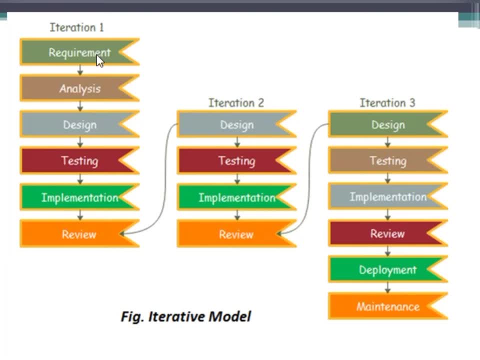 these requirements and on the basis of these requirements we make a requirement document called the software requirement document. We do analysis on the basis of SRS. Analysis is how our requirement should be accepted and how it will work. Based on the analyzed requirement, we prepare a design. 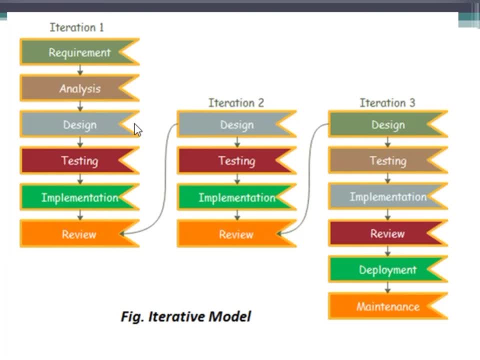 This design can be any form of design which will be suitable to work on by the programmers. It could be DFD, use case diagram, flow diagram, algorithms, anything, And based on these diagrams, we implement the project. We actually start coding and implementing and testing the project. 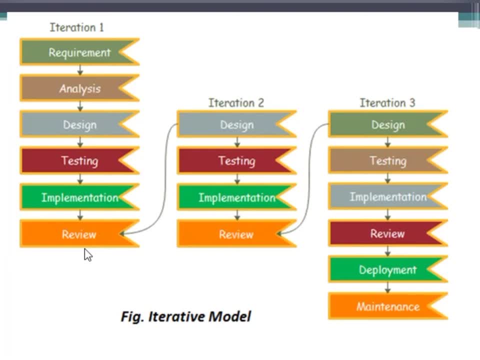 After testing the project, we will have this review phase. In this review phase we review our entire software. We match the requirements. If new requirements come, we accept them too, And on the basis of this reviewed document we judge that we should do the second iteration. 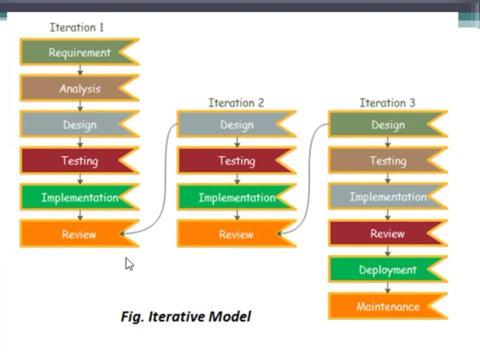 If we want the next iteration, we forward the next iteration with the changes. We will incorporate all the changes in this review And we will send those changes in the next phase or in the next iteration. There will be no requirement analysis in the next iteration phase. 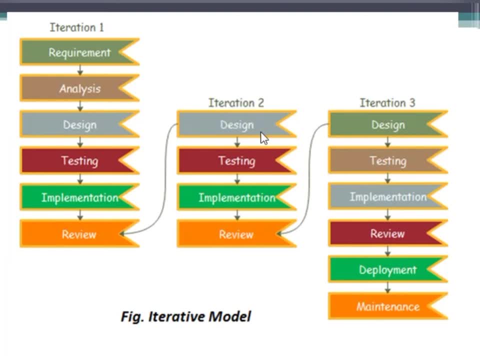 We will start directly with designing. This design will be based on the changes that we have proposed in the previous iteration. Based on all the changes in the previous iteration, a new design will be made. Then again, the same things will happen. We will do testing, implementation and review again. 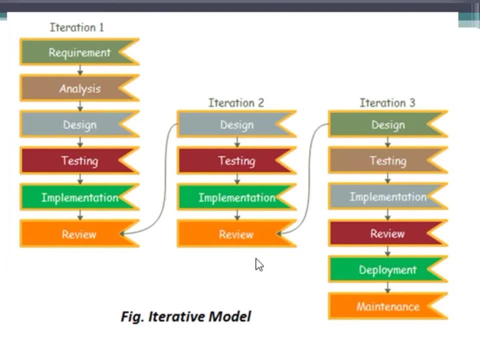 We will conduct this review process until we get any new changes in the review. When we do not get any new changes in the review and our review is accepted, in that case we deploy the project. We deploy means if we are making it for a customer. 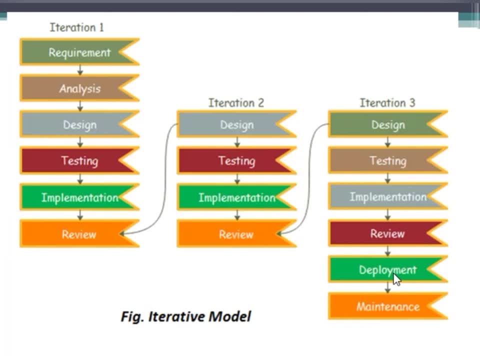 then we deliver that project to the customer. If that product is for the market, then we launch it in the market. After this we have the last phase, which is maintenance. Maintenance is basically software maintenance, where software is continuously monitored, feedbacks are collected and based on the changes, 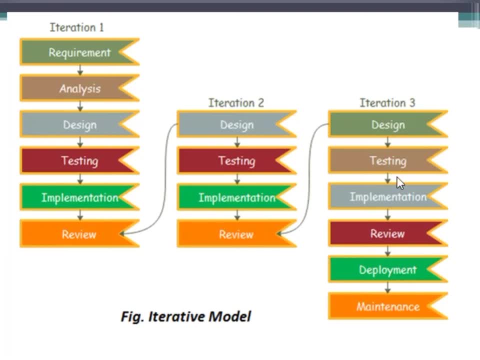 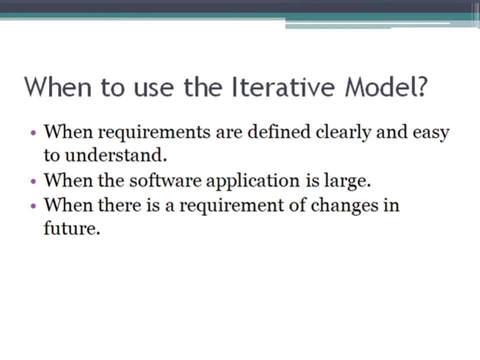 we follow maintenance to resolve the bugs. So this is the working of iteration iterative model. Now, where do we use iterative model? When and where will we use this model? For this, we look for specific points When the software application is very large. 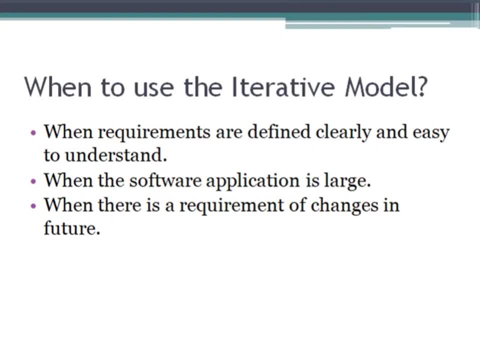 if you are applying multiple iterations, then the benefit will be when the size of your software is very large. If your software is of small size, then multiple iterations will only cost you. Your budget will only increase. This project is suitable only for large applications. 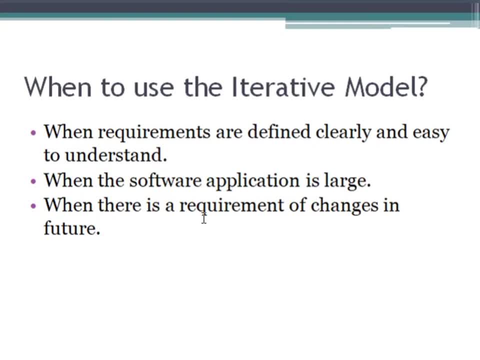 This model is suitable When there is a requirement of changes in future, when you think that there will be changes in your project in the future. that is why we make versions. If you see some software versions come, then we work in the first version. 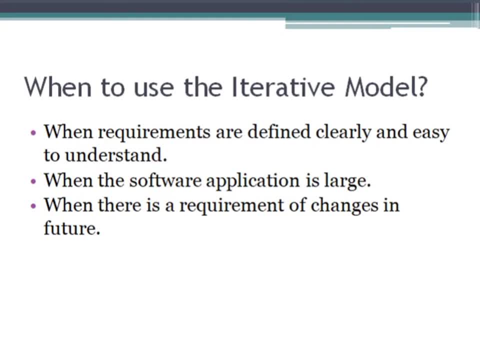 and after two years- three years according to the new changes that come- we start using the new version of the same software. So this is also beneficial for that type of software iterative model And when the requirements are defined clearly and easy to understand. 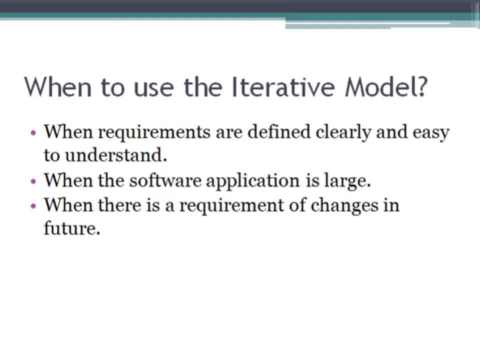 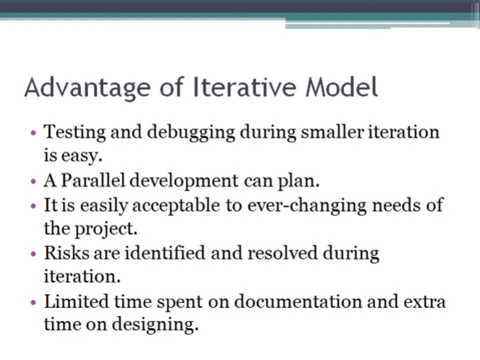 when your requirements are clearly mentioned, then we follow the iterative model. Based on these points, we can say what are the advantages of iterative model. Testing and debugging of iterative model is very easy Because you are making small models, making small iterations. 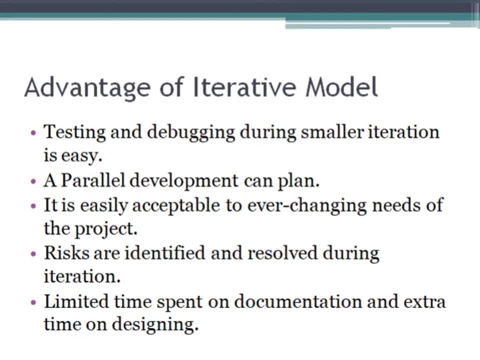 it becomes very easy for you to test or find out the errors. In fact, this is the reason that we can identify the risk quickly and can resolve the risk quickly. So to identify the risk quickly, to resolve it quickly, to do testing or debugging quickly. 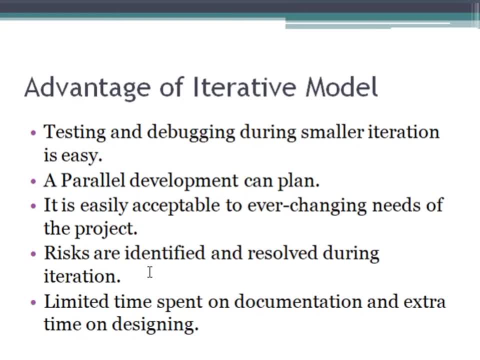 are some of the best advantages of the iterative model. We can use this model for parallel development. Since we are following iterations, then we can work on the basis of iterations or we can execute parallel projects. It is easily acceptable to ever changing need of the projects. 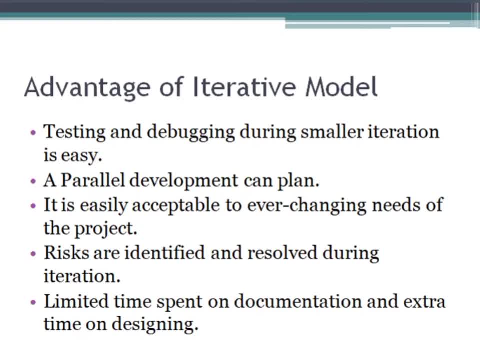 As the changes come in the projects which we refer as versions. for that this model can be used. For that this model is very beneficial. So such large scale projects which after years of span or months of span, want to release a new version, 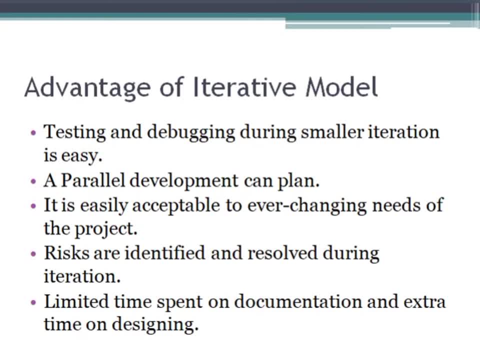 there we can implement iterative models very easily. And last advantage is limited time spent on documentation and extra time on designing. So here we focus more on making the product better compared to documentation. So documentation is less and limited, whereas project is most refined and valuable. 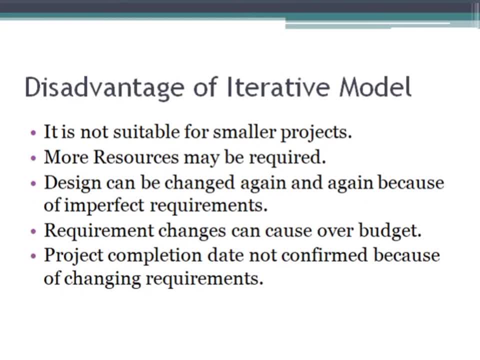 There are some problems with this model which we can consider under disadvantages. It is not suitable for smaller projects. So if I want to take all the advantages but my project size is small, then this is not very fruitful. Right If you are following the iterative model. 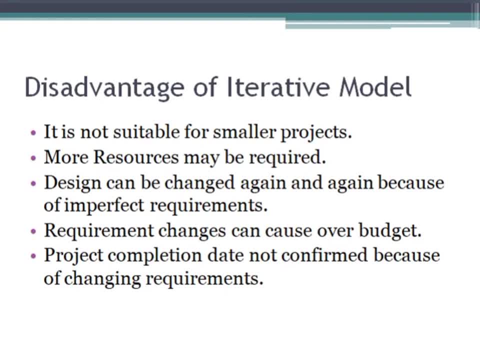 then our resources will be consumed more, Because multiple times iterations are taking place. every iteration requires resources, So we need more resources whenever we are following the iterative model, Designs can be changed again and again because of imperfect requirements, Since requirements are changing again and again. 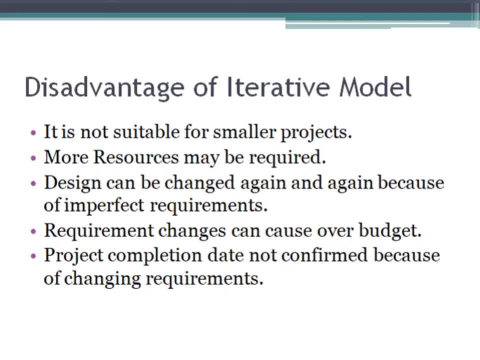 then you have to design multiple times. As we saw in the diagram, each iteration starts with the design phase, So the cost of designing is comparatively high in this model and in comparison to other models. Right Requirements changes can cause over budget. 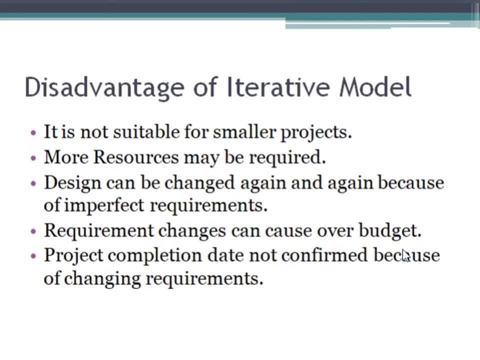 If you change the requirements multiple times, then the possibility of budget exceeding remains in this model. So we try to implement this model in minimum budget so that we can gather the requirements together. Project completion date is not confirmed Since, as we discussed earlier, 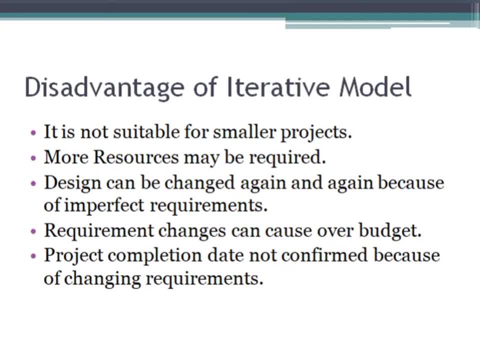 the number of iterations is not certain, We cannot say that to implement this model how many number of iterations will take. Since the number of iterations is not confirmed, then it becomes difficult to tell the due date or end date initially. So these are some disadvantages. 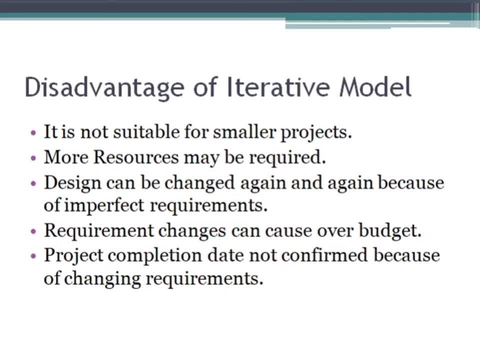 with this model. I hope this lecture will be clear. If there are any problems, then you can ask your queries in the comment section. Thank you.